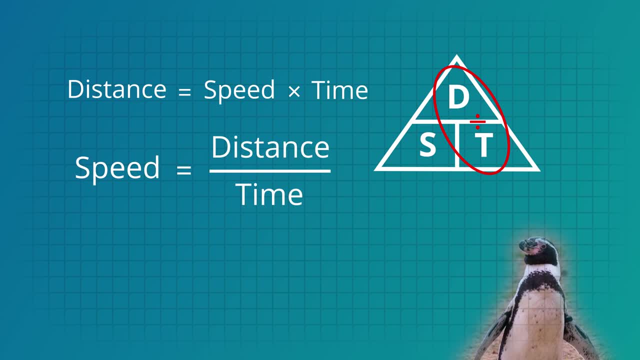 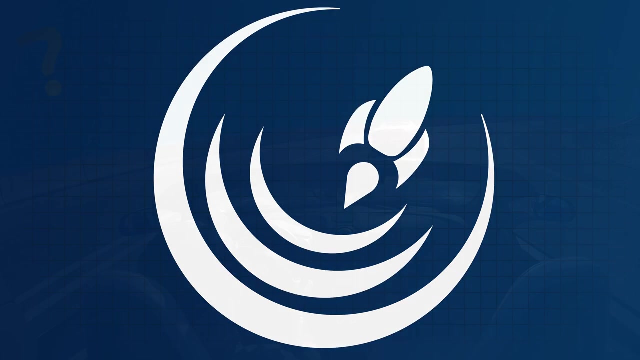 we divide. Speed equals distance divided by time. Now for the third rule: to find the time, Highlight the T in the triangle, Because D is above the S. we'll divide. So the time equals distance divided by speed. Easy to remember. Now let's test you out. Let's find the distance. 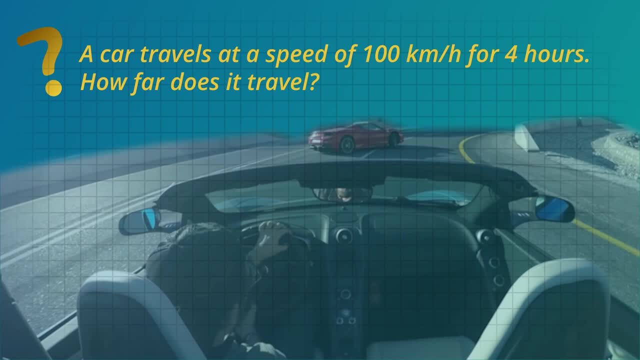 A car travels at a speed of 100 kilometers per hour for four hours, How far does it travel? Hey, remember the DST triangle. Distance equals speed multiplied by time. The speed is 100 kilometers per hour and the time is four hours. So when we multiply them, the distance equals 400 kilometers. 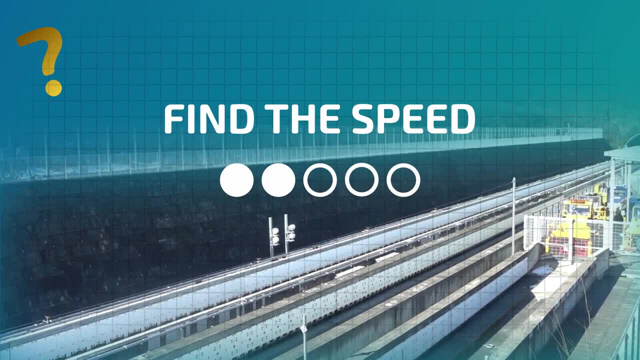 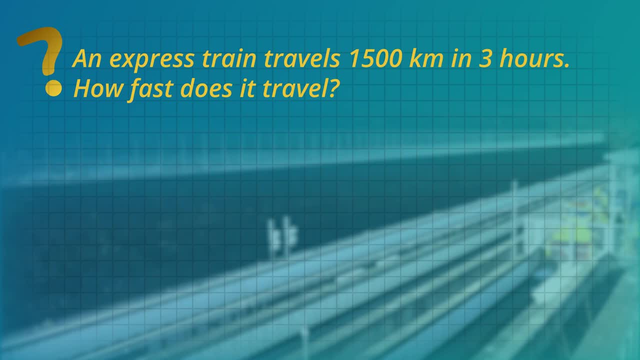 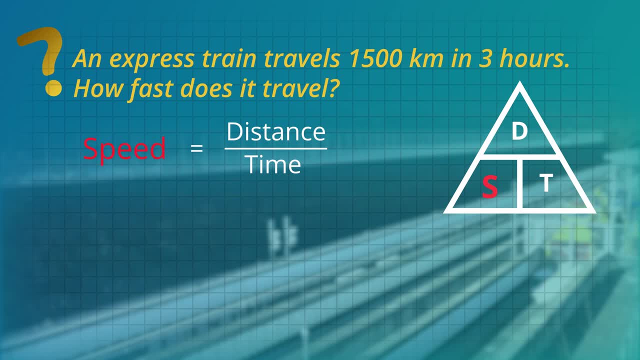 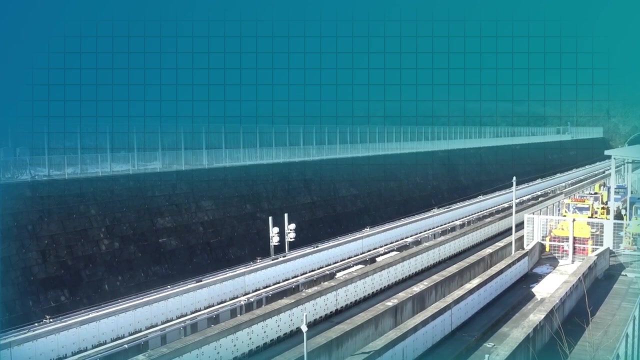 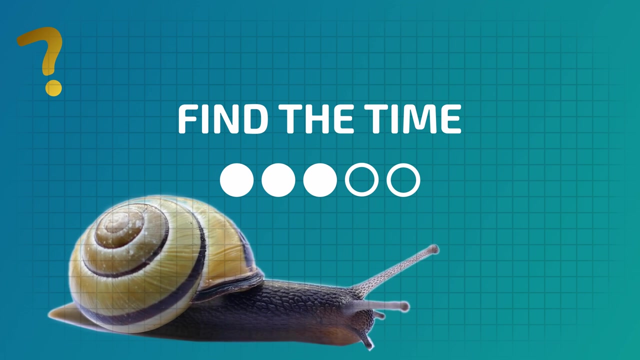 Okay, here's the DST triangle. Speed equals distance over time. We know the distance is 1500 kilometers and we know the time is three hours, So the speed is a super fast 500 kilometres per hour. Now let's do an example to find the time at a snail's pace. 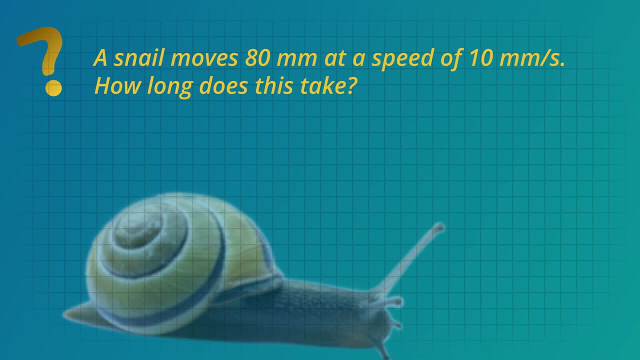 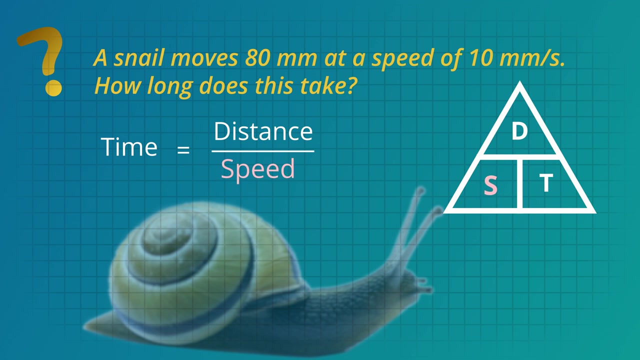 A snail moves 80 millimetres at a speed of 10 millimetres per second. How long does this take From the DST triangle? the rule is: time equals distance divided by speed. That's a distance of 80 millimetres divided by a speed of 10 millimetres per second. 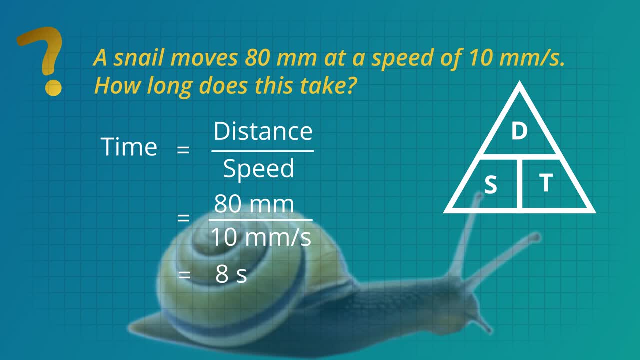 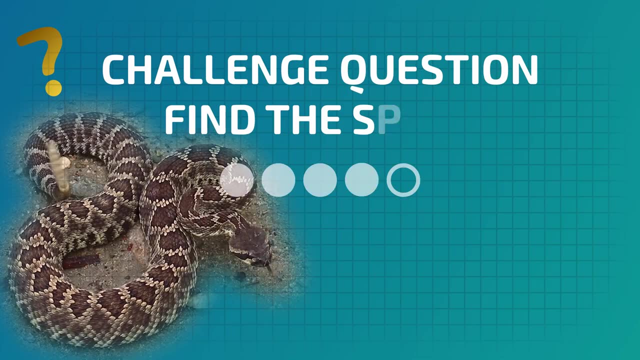 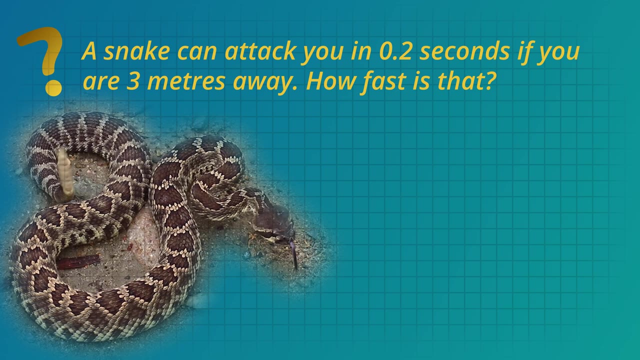 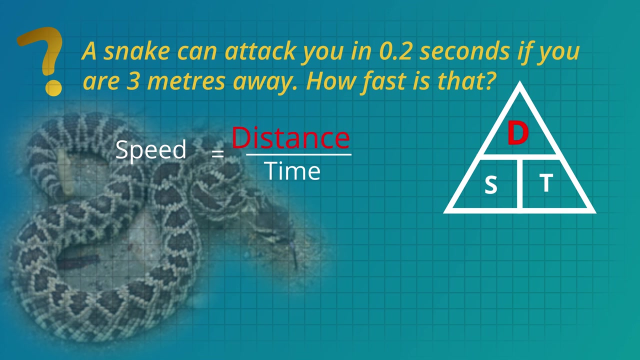 That gives a time of 8 seconds for the snail to slime across my foot. Alright, here's a challenge question. A snake can attack you in 0.2 seconds if you are 3 metres away. How fast is that? Speed equals distance over time.